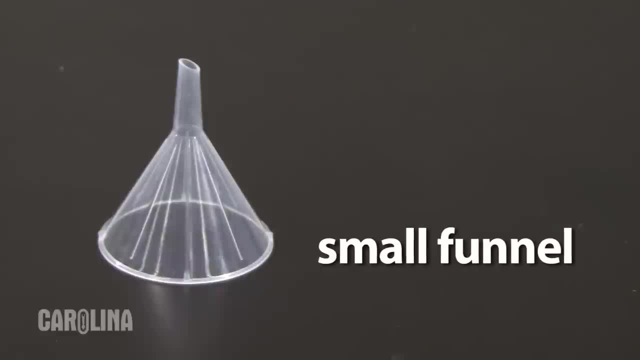 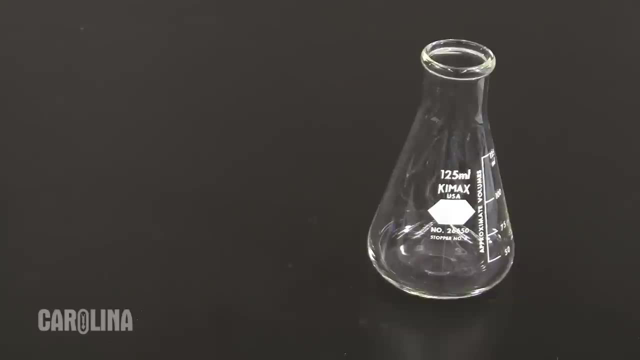 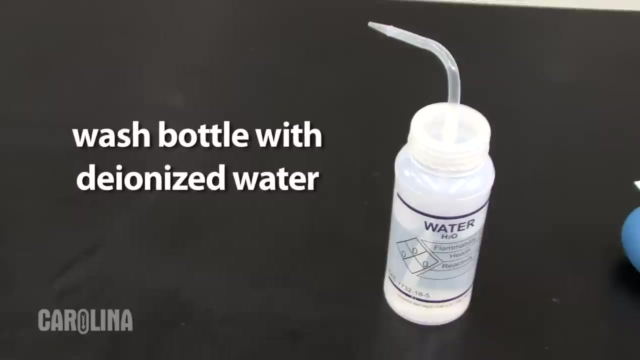 materials you will also need include a small funnel to help you fill the burette, a wheel stopper and a flask. The flask is a 125-milliliter Erlenmeyer flask, which works best for titrations. The shape: 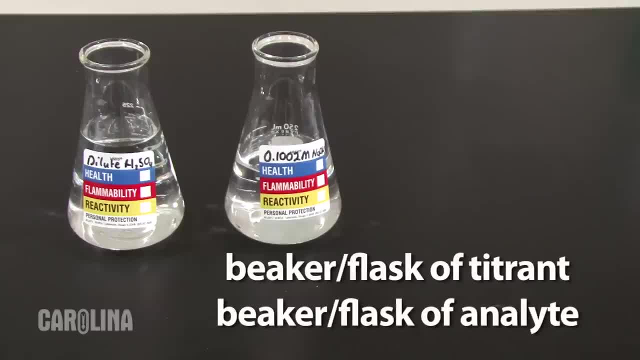 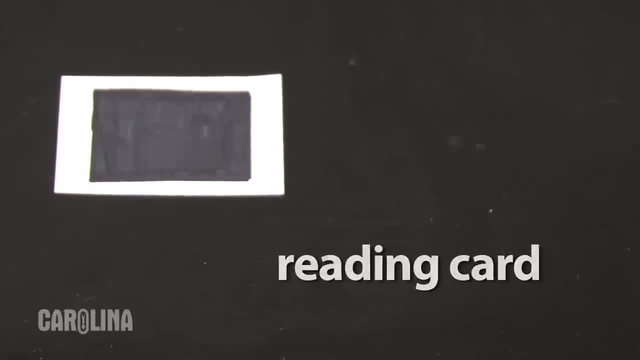 of the flask allows for more vigorous swirling than a beaker or other glassware and minimizes spill hazards. A volumetric pipette and pipette bulb to transfer a known volume of analyte to the flask. A wash bottle filled with deionized water. a beaker or flask of titrant and of. 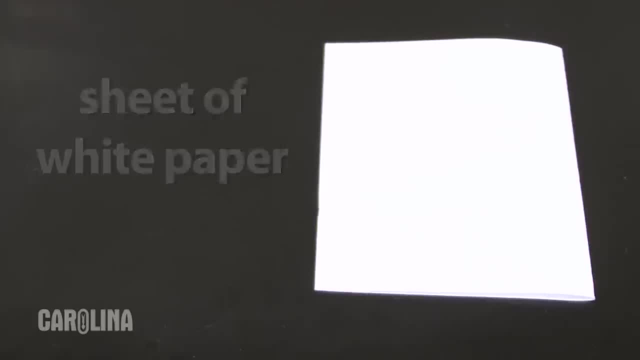 course, a sheet of white paper to help visualize the end point. To prepare your burette for the titration, it is good laboratory practice to rinse your burette thoroughly with deionized water, then with a small amount of titrant After each. 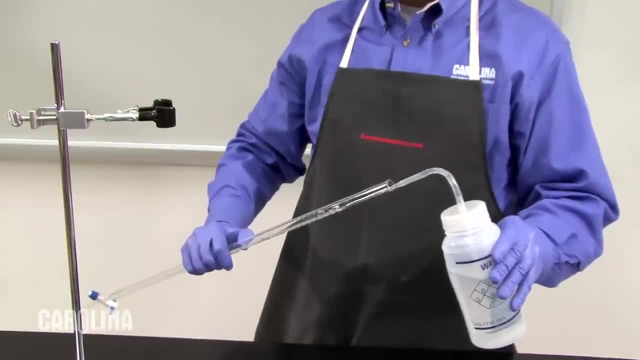 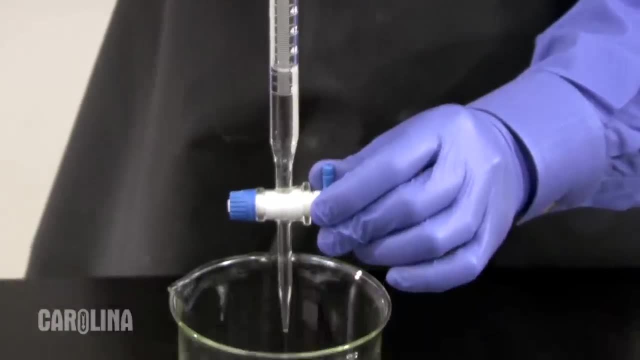 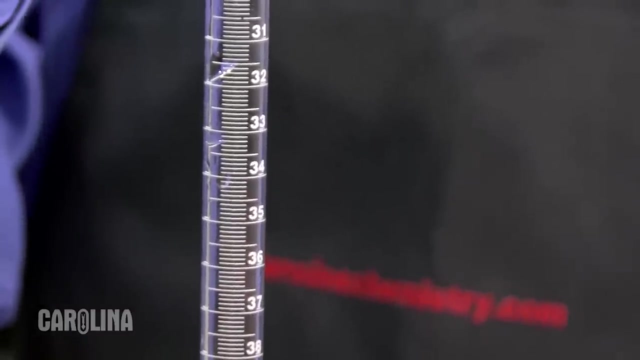 rinse, open the stopcock to allow the liquid to drain out the bottom. If there is a lot of liquid clinging to the walls of the burette, then thoroughly clean your burette and repeat the rinse process. The accuracy of this technique is dependent on the titrant flowing through. 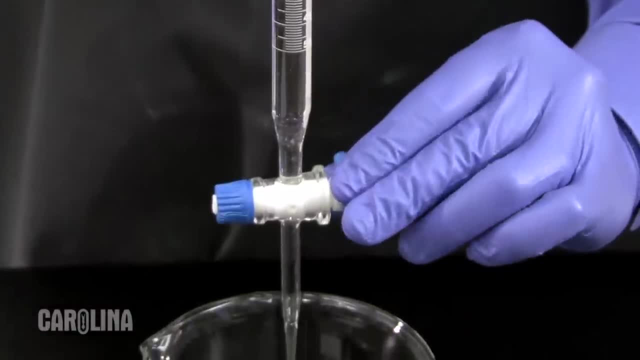 the burette. The flask is a long narrow graduated tube used to add titrant. The flask is a long narrow graduated tube used to add titrant. When we pump water into the flask we should see a slimy groove on the titrant and if it is too hard on the flask we should see. 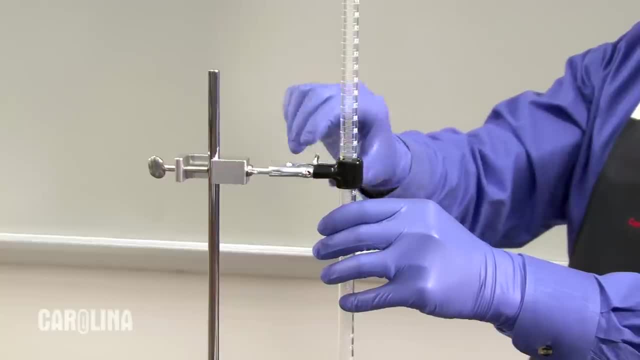 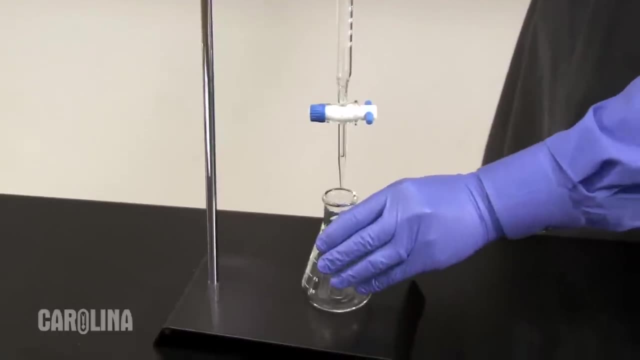 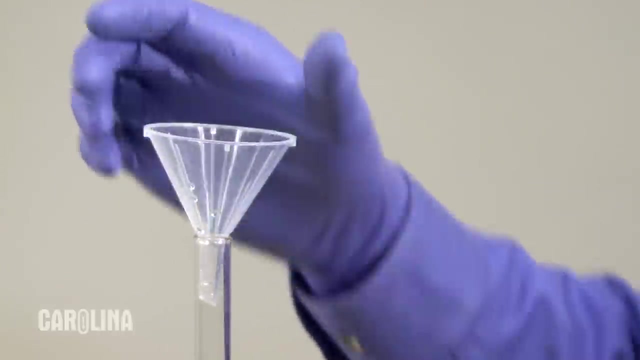 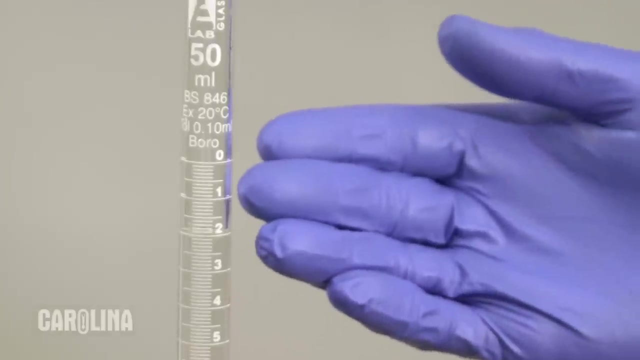 the slimy groove on the burette To make sure this is all leveled out. we want to make sure that the flask is controlled by the tip of the funnel. This is one of the main steps of filling the flask. You may need to use a little bit of a. 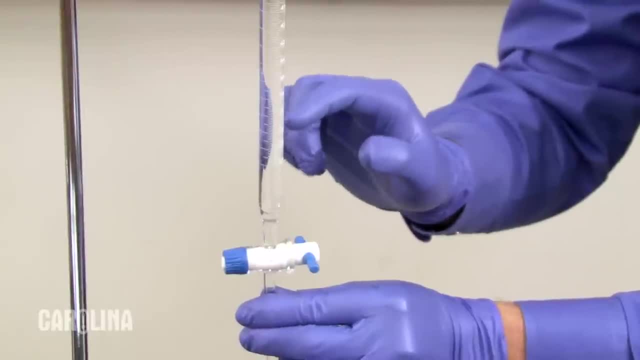 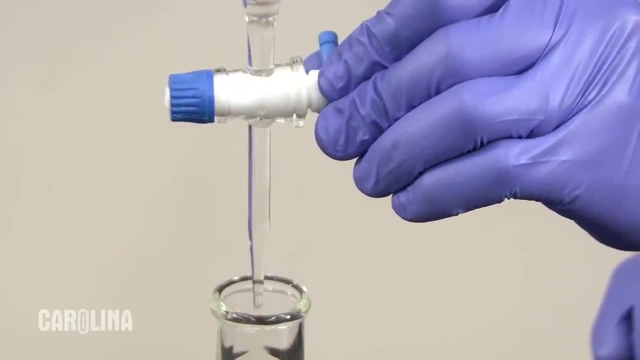 deionized water. Check the column for air bubbles and gently tap to free them from the side walls. Remove the funnel, Place the Erlenmeyer flask under the tip and open the stopcock to allow a few milliliters of titrant to flow through, releasing any trapped air. 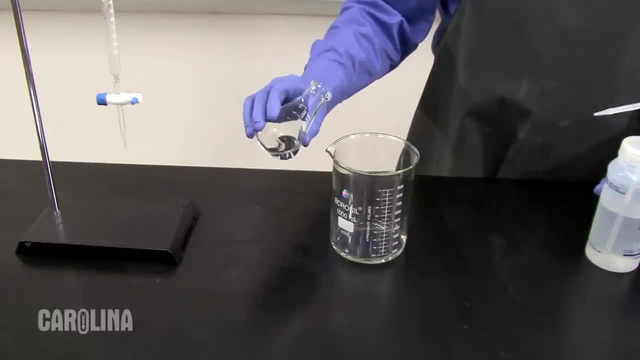 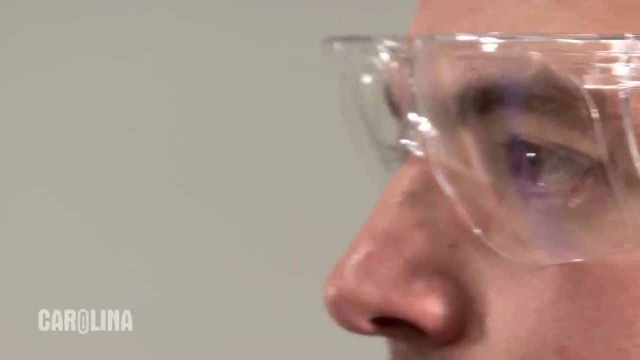 Rinse the tip of the burette with water, Empty the liquid into a waste container and thoroughly rinse the flask. It is not necessary to dry the flask. Record your starting volume. It is important to accurately read the volume on the burette. 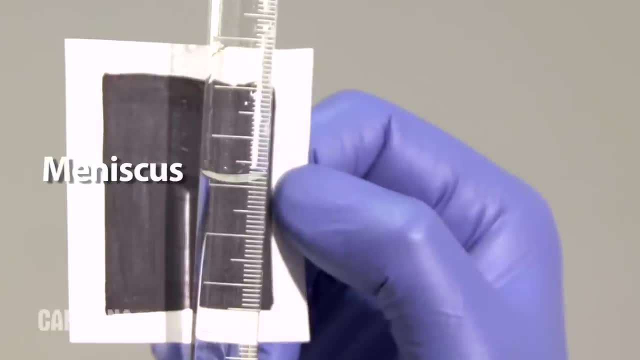 First note that the liquid forms a concave meniscus because the water pulls itself up the side walls of the glass. You should read the volume from the bottom of the meniscus at eye level. Secondly, it is important to read your volume to the correct number of significant figures. 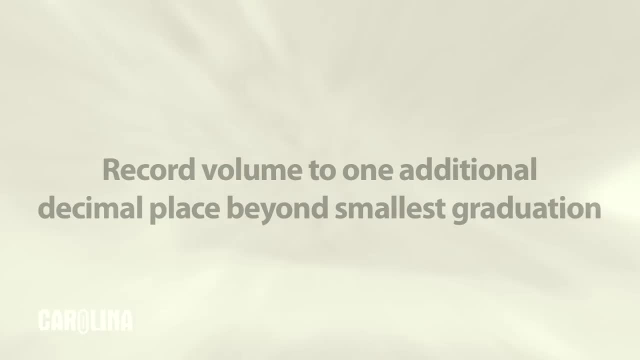 This burette indicates volume to the nearest 0.1 milliliters. With any graduated glassware, record the volume to one additional decimal place before you place the flask into the flask. In this case, record the volume to the nearest hundredth of a milliliter, estimating the 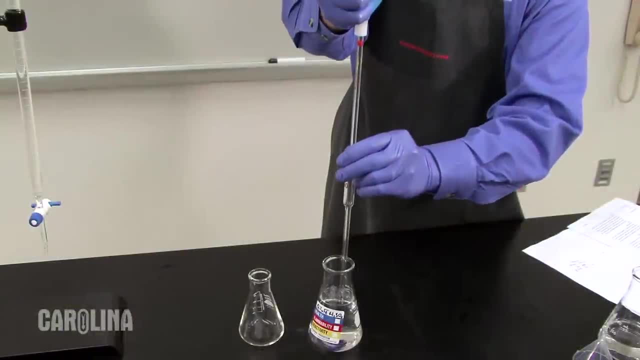 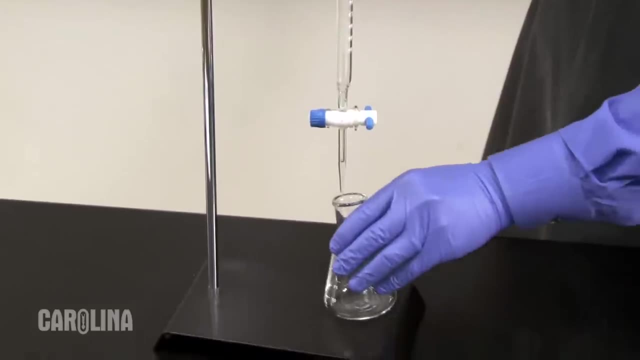 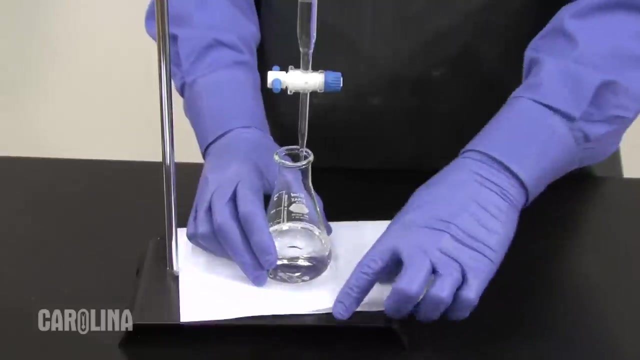 final place, Use the volumetric pipette to transfer the analyte to the flask. Add a few drops of indicator to the flask and swirl. Place the flask under the tip of the burette. Record this volume. Placing a piece of white paper under the Erlenmeyer flask may make it easier to detect the color. 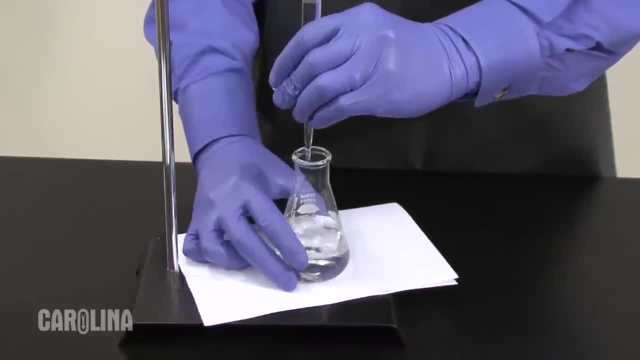 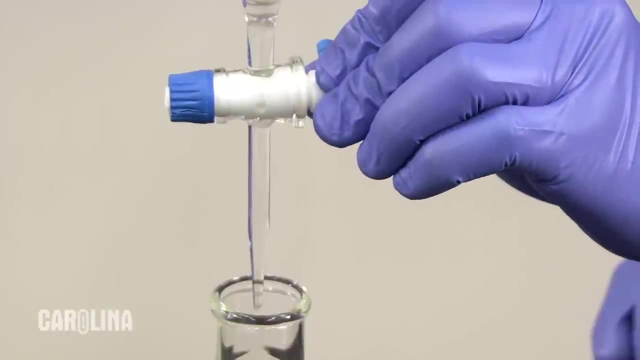 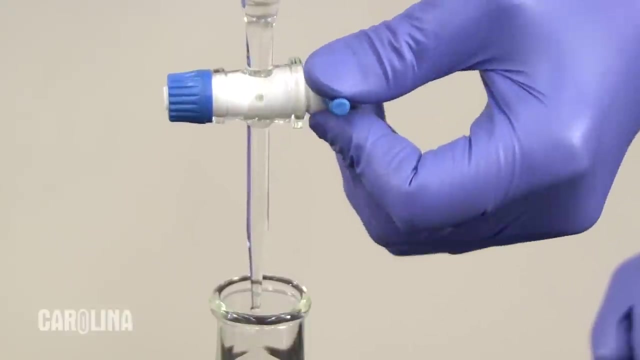 change. Operating the burette requires two hands. One hand turns the stopcock, while the other hand swirls the flask. Practice turning the stopcock a few times to familiarize yourself with how quickly the flow starts and stops. It is common laboratory practice that the first titration is an estimate. 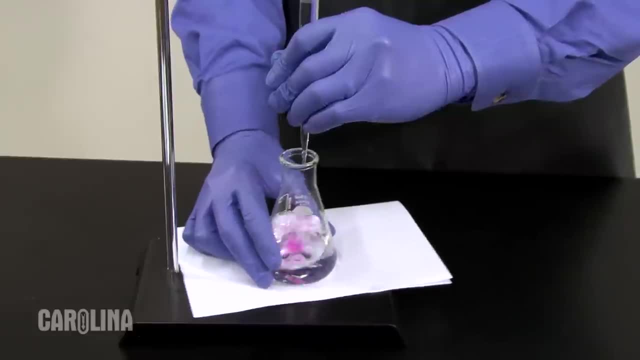 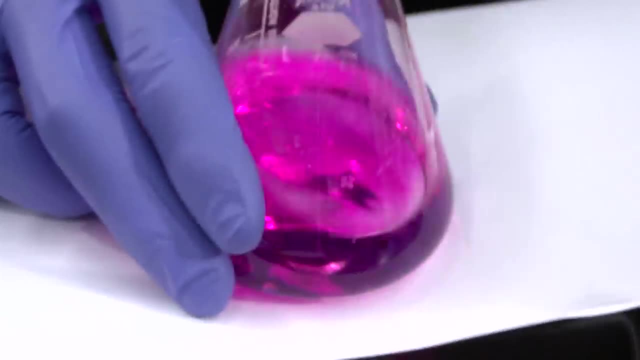 Open up the stopcock and allow the titrant to enter the flask quickly. Continuously swirl the flask. As the volume of titrant in the flask increases, the color of the indicator appears then disappears as you swirl. When the analyte becomes a colored stopcock, the flask is ready. 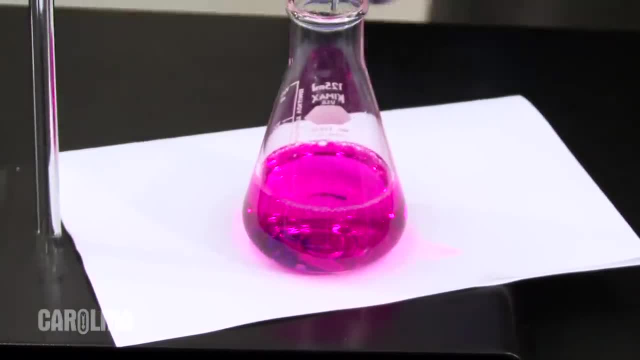 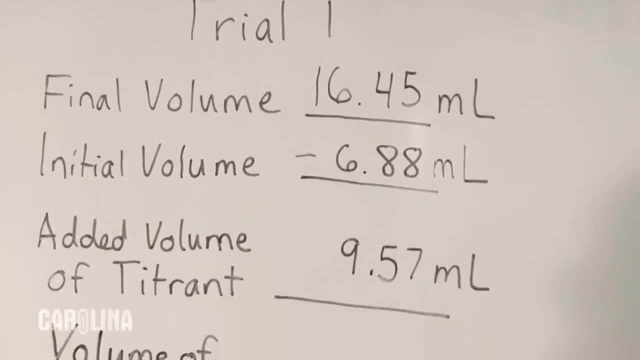 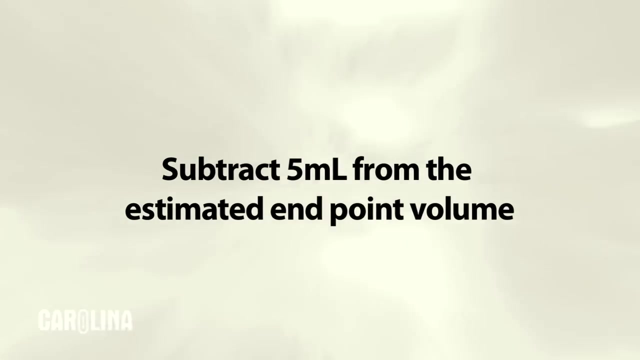 When the analyte becomes a colored solution. close the stopcock. Record the final volume of the burette. Subtract the initial volume from this final volume to get the estimated volume of titrant needed for this titration. Knowing the volume that is a little past the end point, subtract 5 mL from that number. 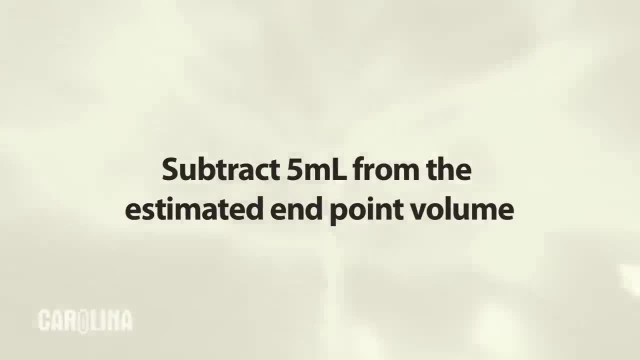 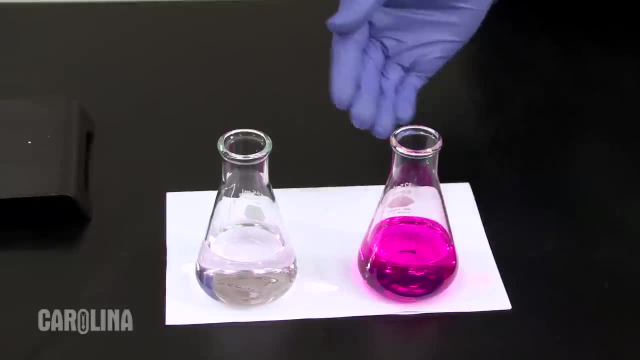 to get the amount of titrant that can be safely added before a slower addition is required. As the estimate titration shows, a dark colored solution indicates an excess of titrant has been added. The desired end point is a pale, faintly colored analyte. 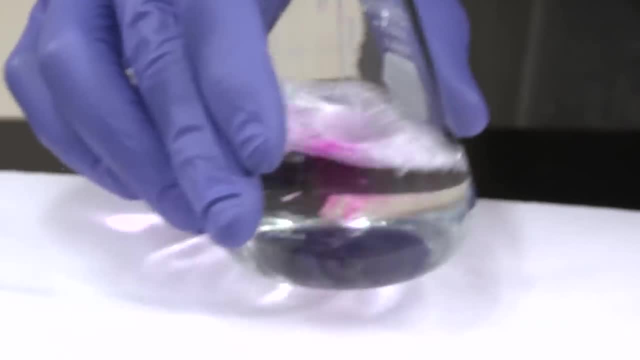 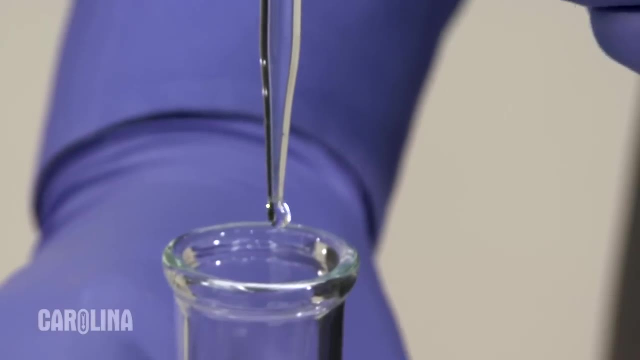 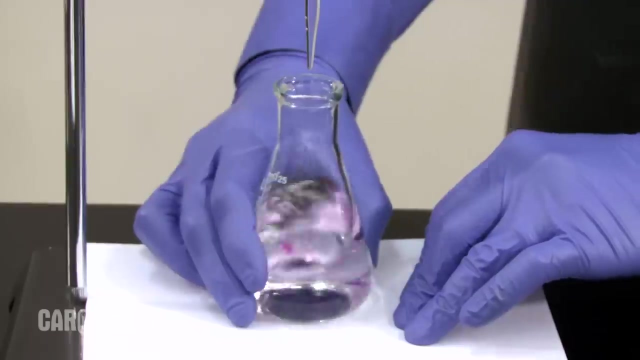 To reduce the risk of passing the end point. slow down the addition of titrant when flashes of color begin to appear in the analyte. Adjust the stopcock to slow the flow of titrant to a drop-wise rate. Continue to swirl the flask with one hand and keep the other hand ready to close the.